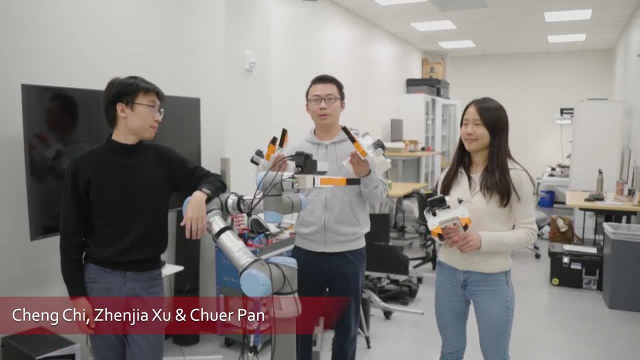 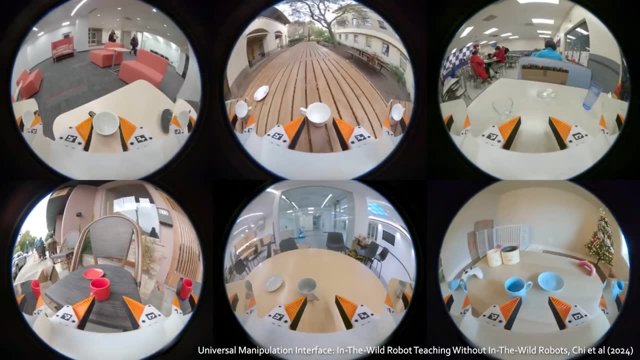 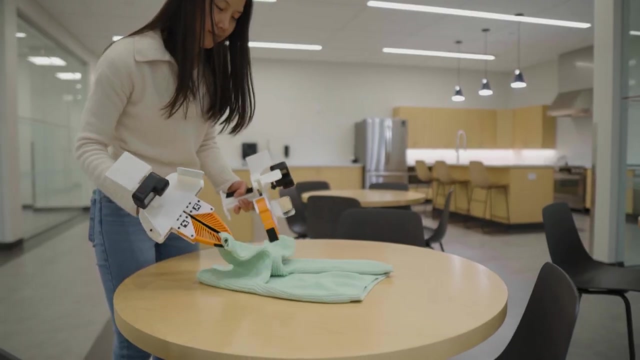 I'm Chou, I'm Linjia, I'm Chuer. We develop universal manipulation interface, A low-cost portable device that allows large-scale in-the-wild demonstration data collection. We can teach robots to autonomously wash dishes, cause objects, book club- all with just a few hours of data demonstration. 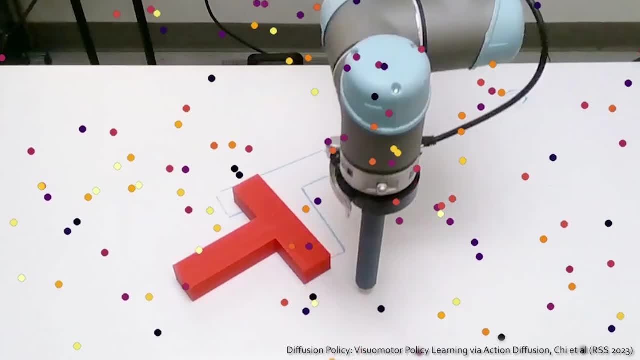 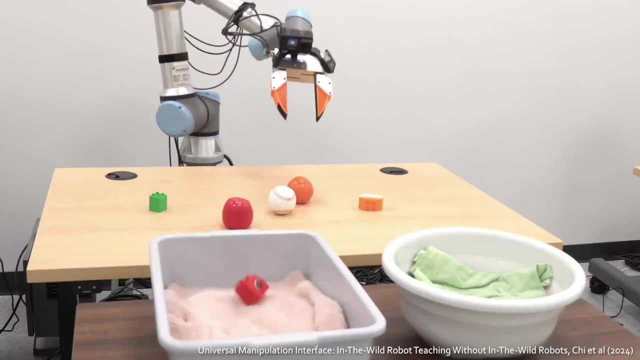 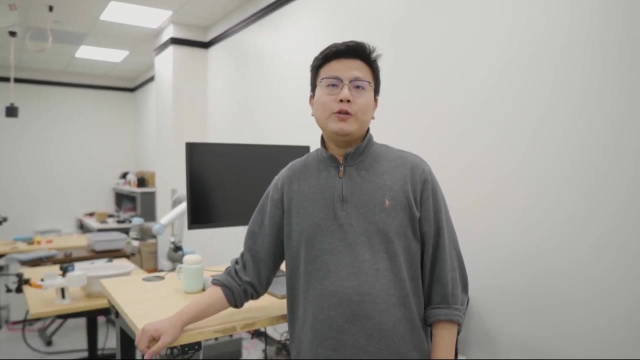 To enable these unprecedented capabilities, we develop diffusion policy, an end-to-end learning framework that captures complex, multimodal human actions. Hi, I'm Minda. Beyond single-scale policy, we develop XQ, which automatically discovers reusable skills such as grasping clothes and opening a microwave, and composes them together to complete non-horizontal tasks. 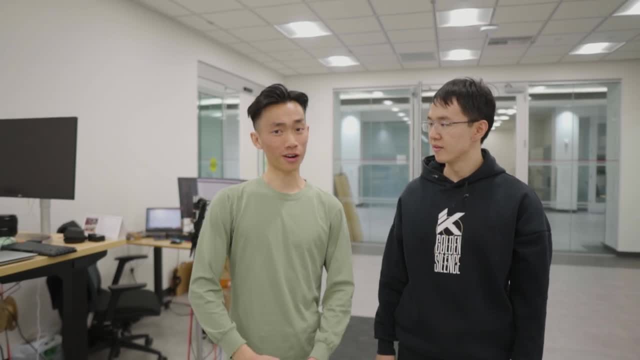 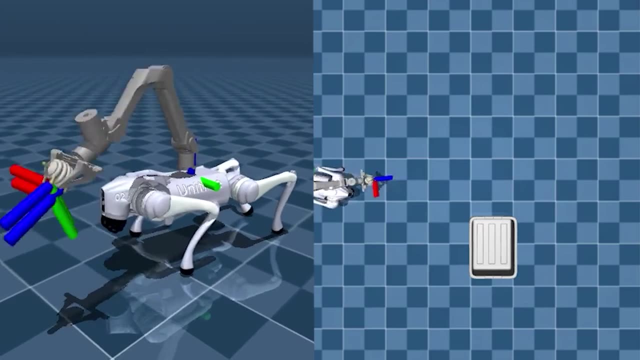 Behavior. cloning is great for tasks that humans are good at, But what about ones that humans aren't good at, such as walking on four legs? In this case, we need a different way to collect robot experiences, such as through the usage of simulators. 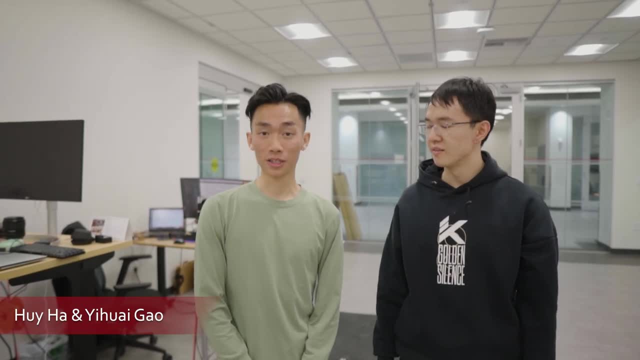 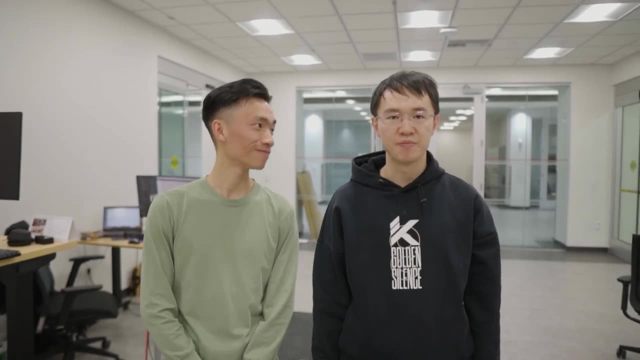 I'm Hui And this is Yihuai, And we're working together to teach robot dogs how to use their entire bodies for manipulation tasks such as grasping, tossing and pulling. To tackle this problem, we train a full-body controller inside the simulator through very cheap trial and error. 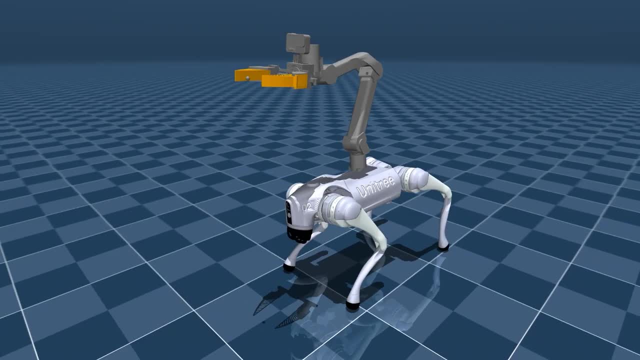 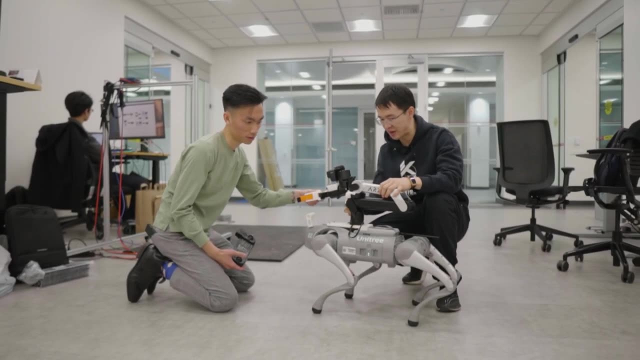 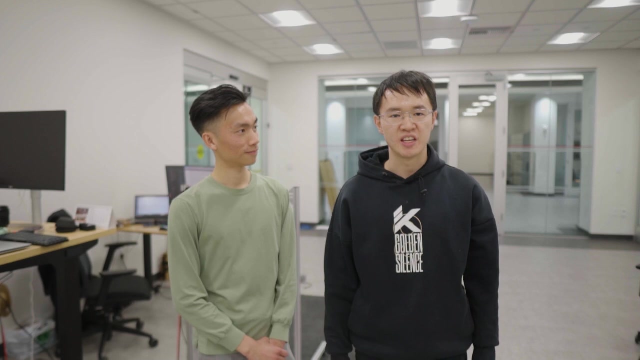 so that the dog gradually learns how to balance, walk and reach. We transfer the learned knowledge from the simulator to the real-world robots And finally the whole-body controller can handle all the movements, given only the ineffective trajectories. This allows the dog body to be included in complex manipulation tasks. 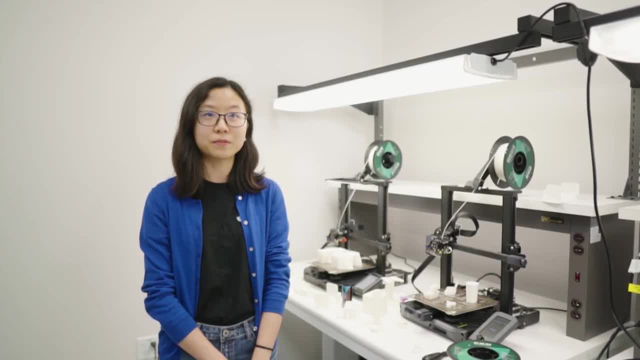 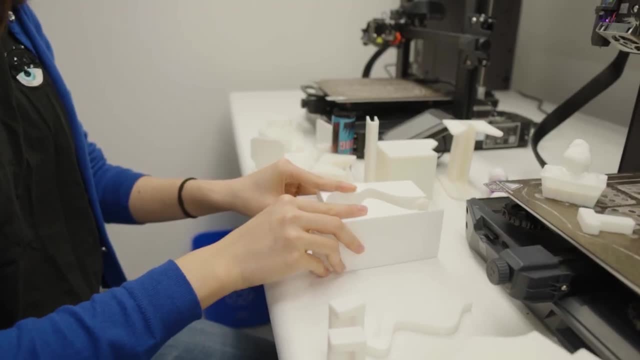 We've seen incredible progress in robots performing different tasks because of Shake's embodiment, But can we generate different robot mechanism designs to adapt to new tasks and environments? I'm Xiao Meng And in our recent work, Dynamics Guided the Fusion Model for Robot Manipulator Design. 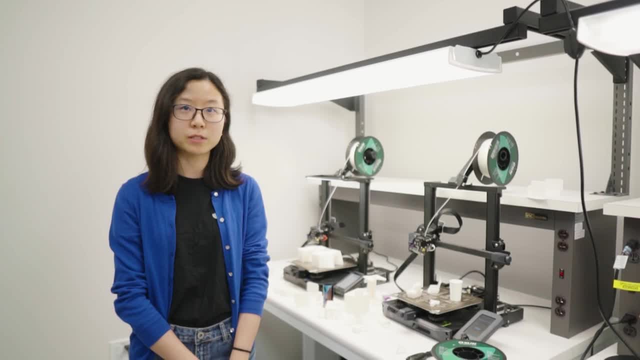 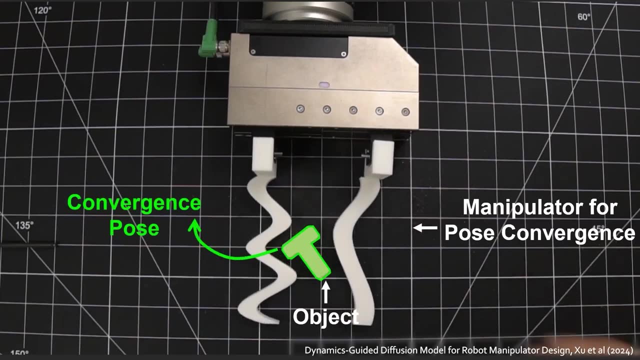 we proposed a data-driven framework for generating manipulator geometry designs, And we also used the platform to generate robotic hands for given manipulation tasks. Our generative manipulators robustly perform drastically different tasks with only an open-loop parallel draw-closing motion and no perception. 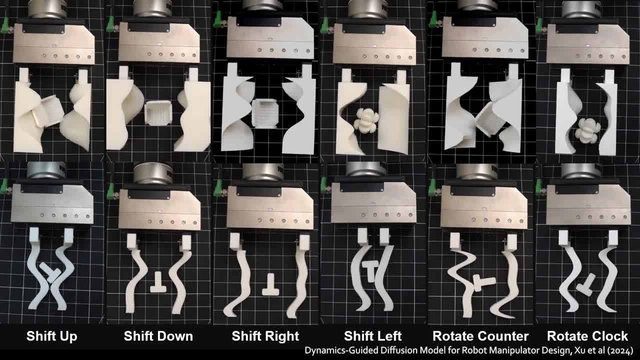 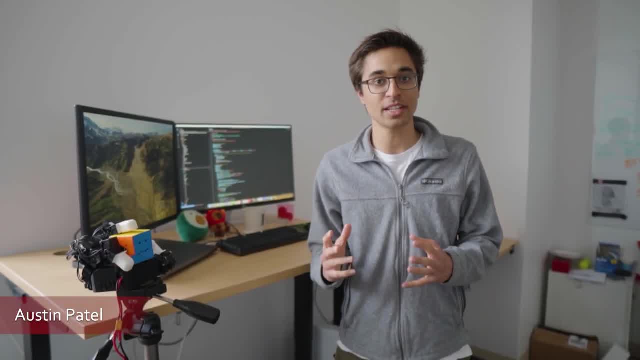 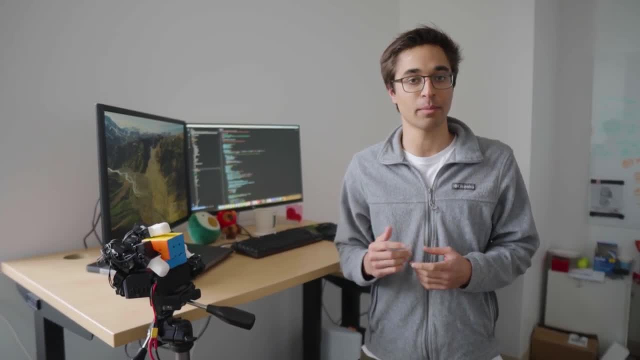 The best part is we generate all of these designs for different objects and different tasks with the same model. Hi, my name is Austin and with the recent advancements in generative robot design, there's an increasing need for robot policies that can generalize across a range of different embodiments. 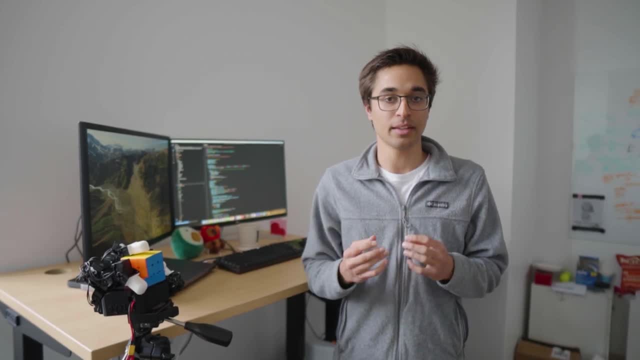 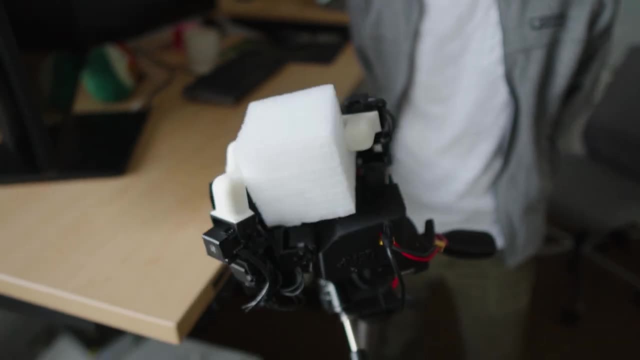 Consider this robot hand. It's a multi-fingered robot hand that has different joints and fingers that can be added or removed, and right now we have to train a separate policy for each of these different configurations. This is costly and expensive and oftentimes really redundant. 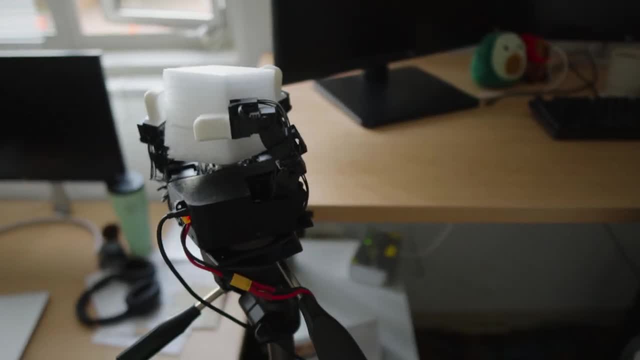 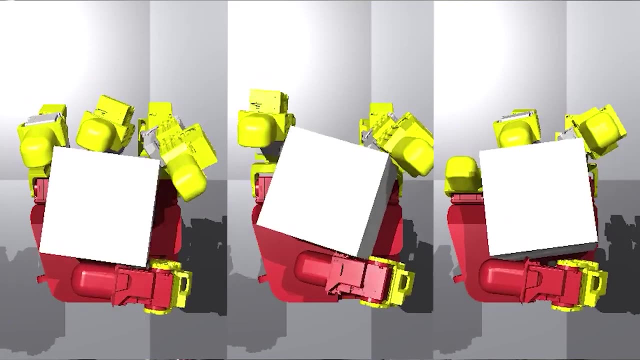 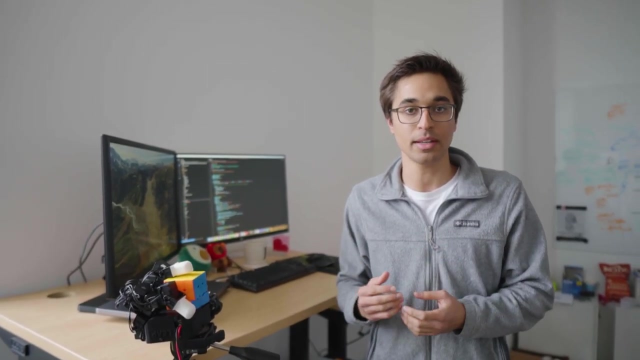 I'm creating a new robot policy that can condition on the current hardware configuration of the robot in order to control it, regardless of whether fingers are added or removed. With this new policy, we're able to have a shared behavior model that can control many different configurations of the hand and even generalize to a brand new embodiment that it hasn't seen before. 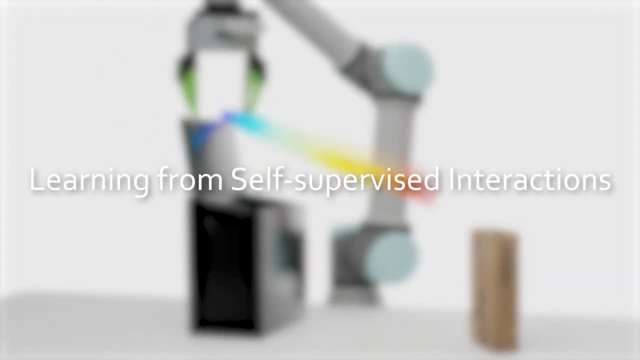 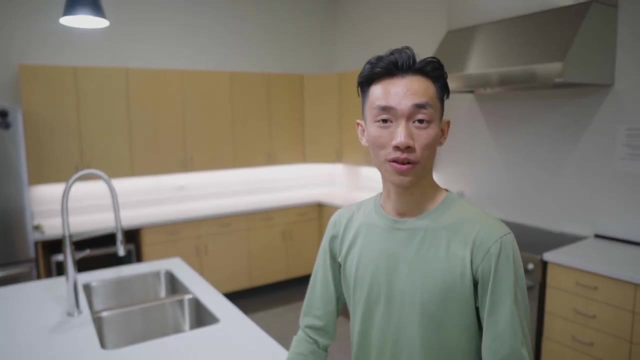 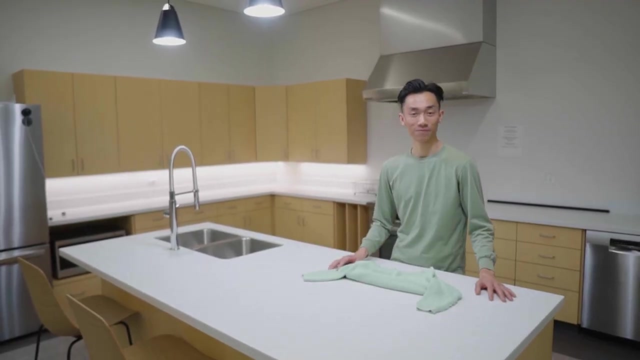 all while training completely in simulation. Now, simulators are great when they're an accurate reflection of the real world, but in some cases that might still be challenging. For instance, simulating cloths accurately is still very challenging. In those cases, we might want a robot to automatically collect its own experiences. 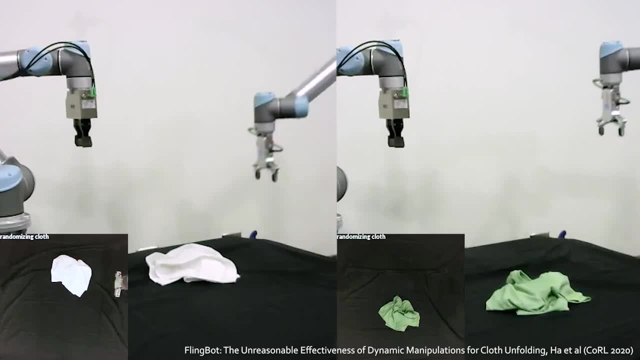 directly in the real world. We've explored this a lot in the past and we're excited to see what we can do with it. We're excited to see what we can do with it In Flingbot, a system that automatically learns to unfold cloths by itself. 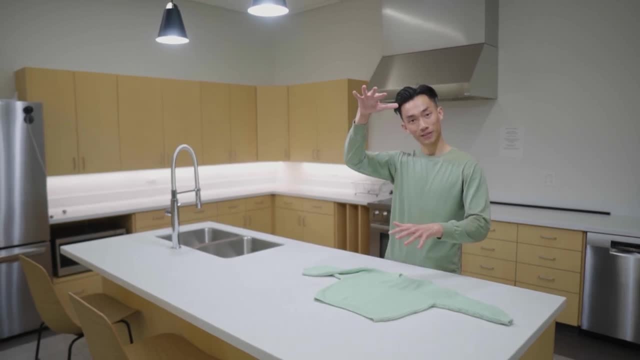 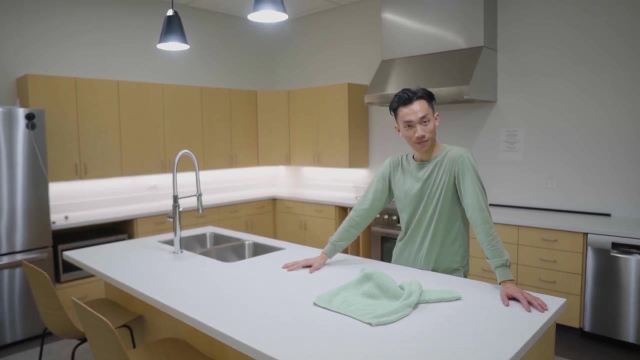 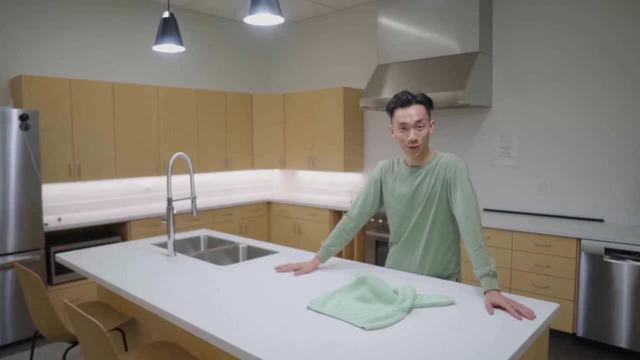 By giving it a top-down camera to track unfolding progress and a mechanism for resetting the cloth after a few unfolding attempts. the system learns by itself. This means I would start the learning process, go home and sleep and in the morning I'd wake up to a system that has learned to unfold cloths. 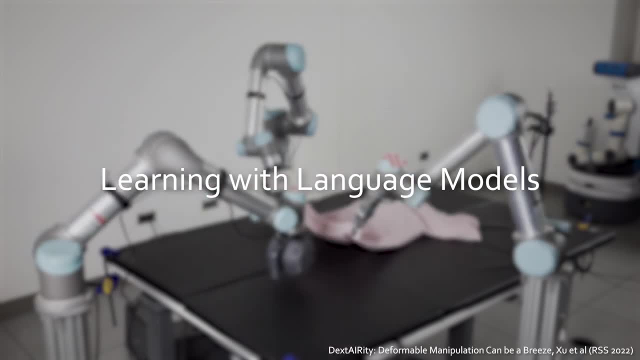 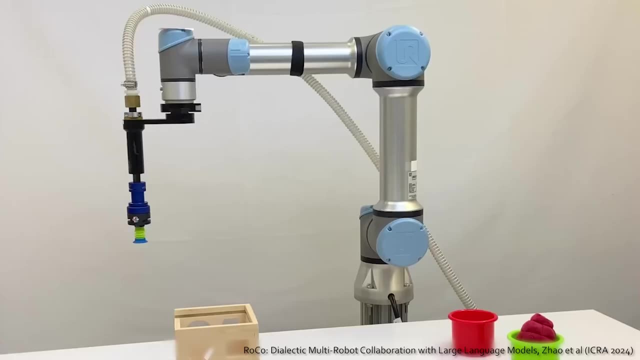 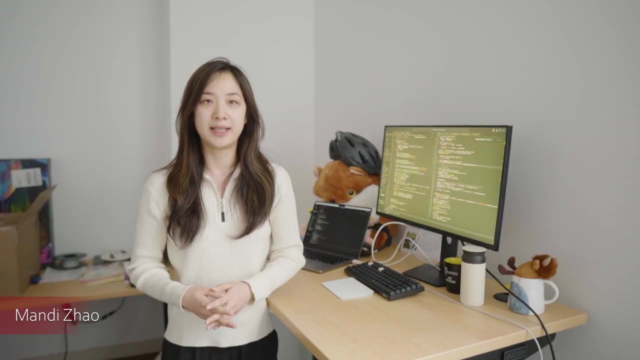 Flingbot is one example where two robot agents have to work together to complete the task. In the real world, many scenarios require robots to collaborate with other agents and achieve more semantically complex tasks. My name is Mandy. In our recent work, Rocko, we study how to use 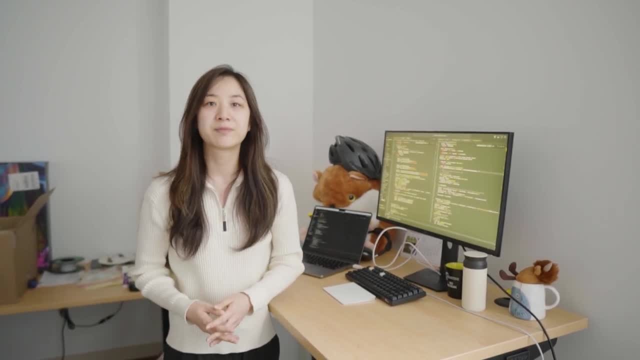 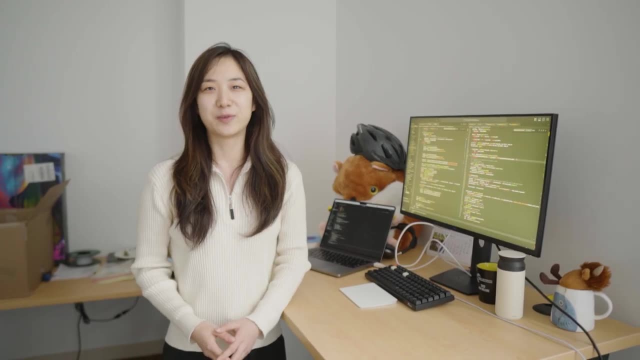 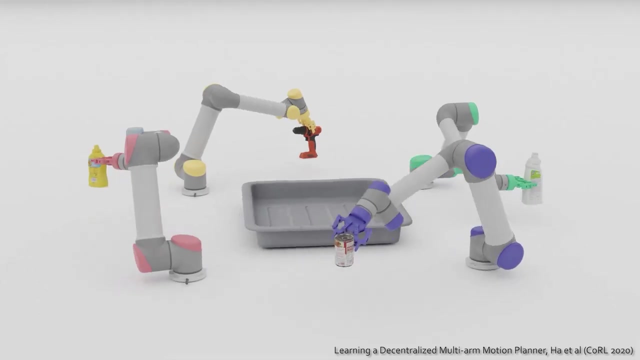 pre-trained large language models. to facilitate such collaborations, We propose a new framework where different agents can discuss task strategies using large language models. We show that this framework can achieve a variety of multi-robot manipulation tasks and we can have a robot talking with a human in real time to complete the task together. 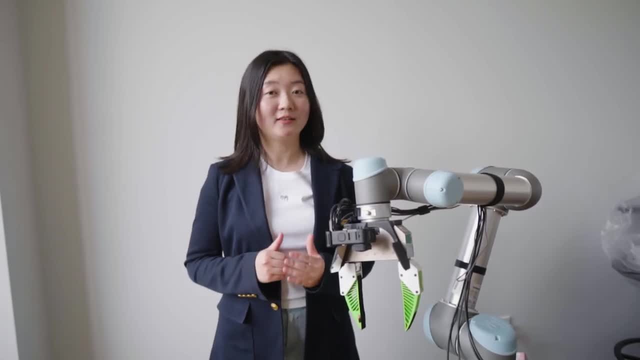 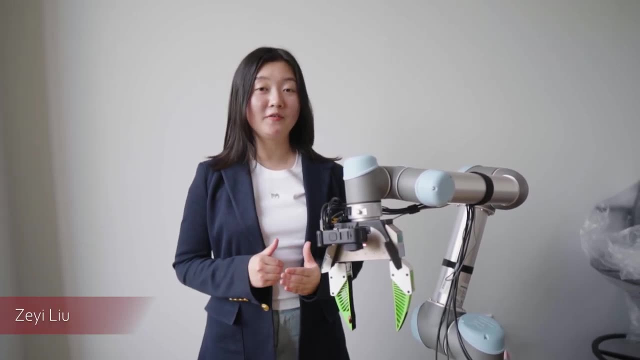 Even though our robots become more capable of handling complex and long-horizon tasks, they still fail a lot of times. My name is Zeyi. In our recent work Reflect, we give our robots self-reflection ability to automatically identify and explain its failures.